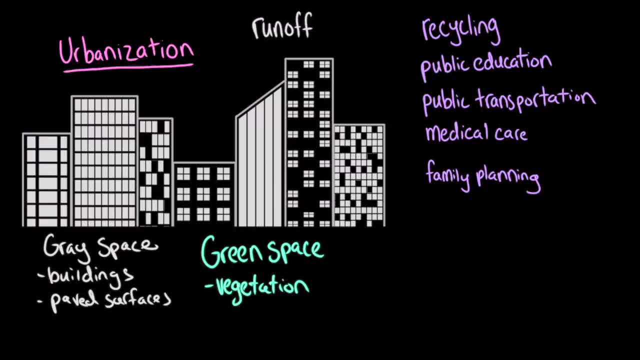 Having nowhere to go, the water travels across the paved surfaces, picking up pollutants along the way. All this runoff can lead to flash flooding. Adding more green spaces can help prevent this from happening, because plants soak up water. There are many creative ways that urban planners can add green spaces to our environment. 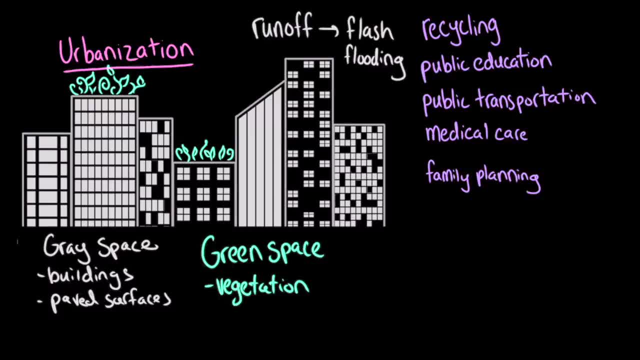 Some buildings and cities grow plants on their roofs. They're called green roofs. The plants soak up the rain and snowmelt that hits the roof and prevents it from going into the street. Also, plants create shade and help cool things down. so buildings with green roofs wouldn't have to spend. 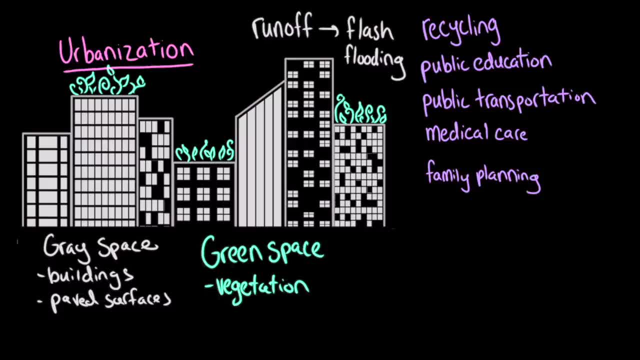 as much energy on air conditioning. Green spaces can also help the environment by allowing for groundwater recharge, which is allowing more water to sink back into the ground and replenish the aquifer. Some cities do this by building rain gardens, which are gardens specifically designed. 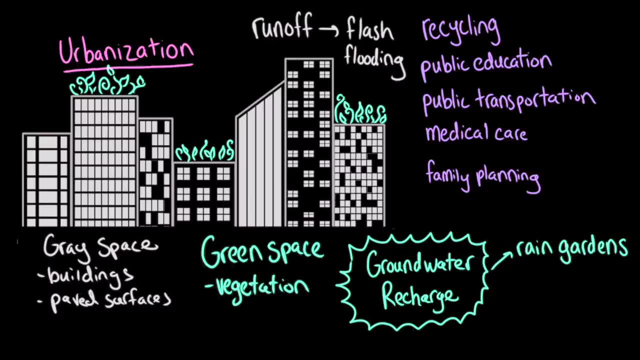 to filter water back into the ground. The plants in the rain gardens help filter pollutants in the runoff and prevent the pollutants from contaminating water ecosystems. Cities can also help with groundwater recharge by building permeable surfaces in their cities. Parking lots can be constructed with permeable paving to reduce runoff. Groundwater recharge can help prevent. 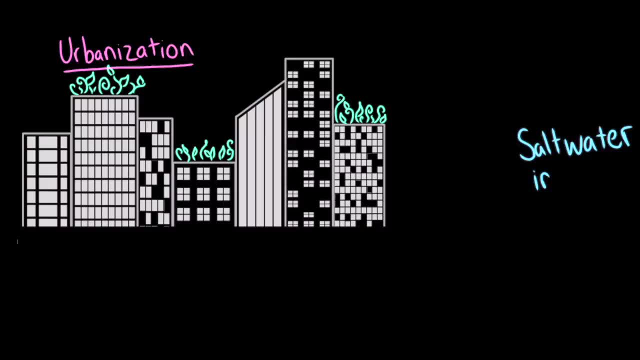 something that happens in coastal cities called saltwater intrusion. Let's say that this city right here is a city on the coast, so it's really close to the ocean. And let's say the city decides to build a pump right here to access the fresh water in the aquifer below it. But the city has a 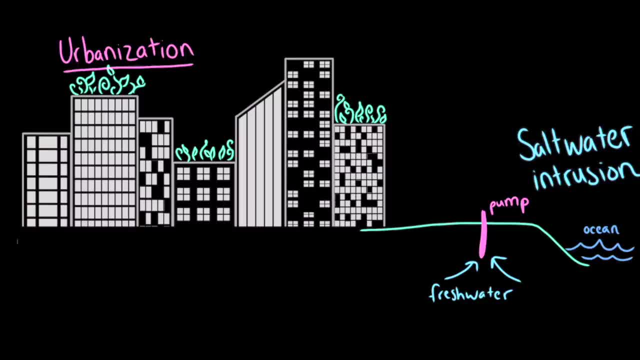 lot of people in it and it needs a lot of water. The city might end up taking more and more fresh water at a rate too fast for the fresh water in the aquifer to replenish itself. Pulling up so much fresh water can create a space for the saltwater in the nearby ocean to come and take. 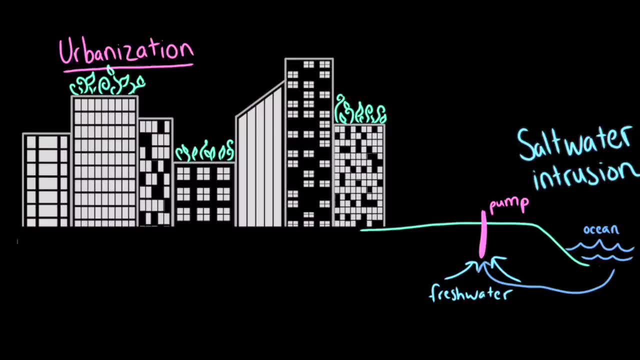 its place. The saltwater from the ocean would contaminate the fresh water supply, making it unpotable. But if this city decided to increase the amount of permeable surfaces and green spaces, then when it rains, the water will be able to seep back. 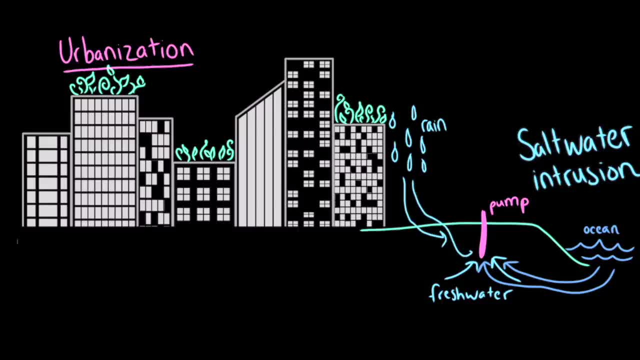 into the ocean, And it would refill the empty space the pump has created with fresh water. This would mean that fresh water would continually be replacing the water that was taken out by the pump, so saltwater intrusion couldn't happen. Adding more green spaces could also help with. 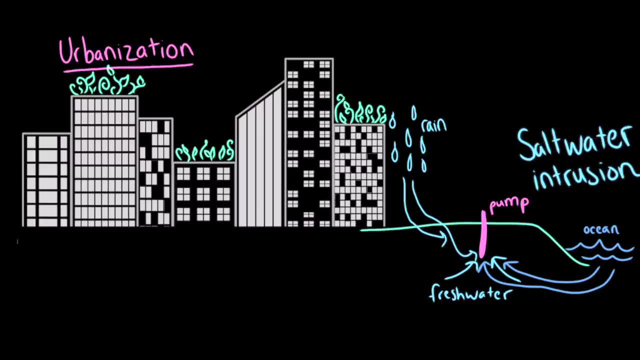 air pollution because plants absorb carbon dioxide and produce oxygen. Cities produce most of the world's air pollution. Part of this is because of urban sprawl. As cities become more populated, they expand into suburban areas And even if you have a lot of green spaces, you can. 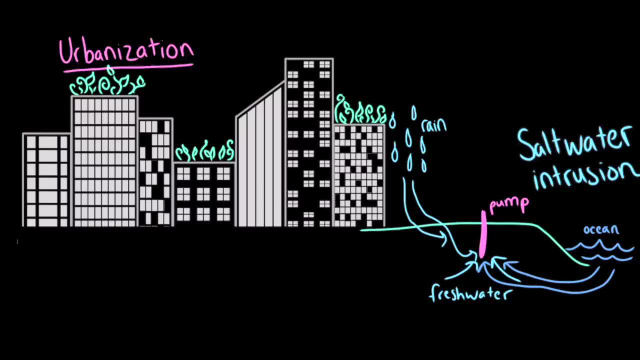 see the green areas of the suburbs. All of that expansion leads people to live farther away from their jobs. This causes people to spend a lot more time in their cars on their long commutes to work, And these long lines of cars of people traveling to work emit a lot of carbon dioxide. 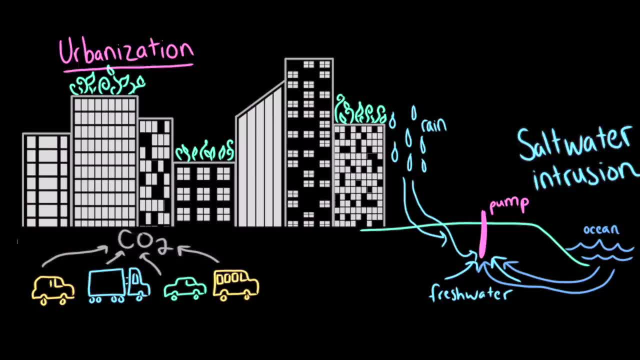 Carbon dioxide is a greenhouse gas, which means it retains heat from the sun and it contributes to climate change. But carbon dioxide isn't the only kind of air pollution that cities produce. Emissions from motor vehicles and industrial facilities in cities can create something called photochemical smog. This is a kind of hazy, smoky pollution that you can sometimes 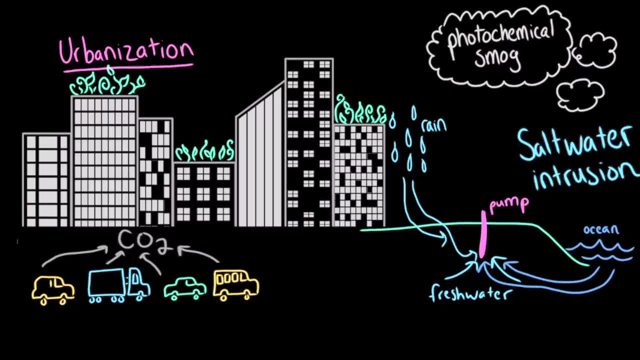 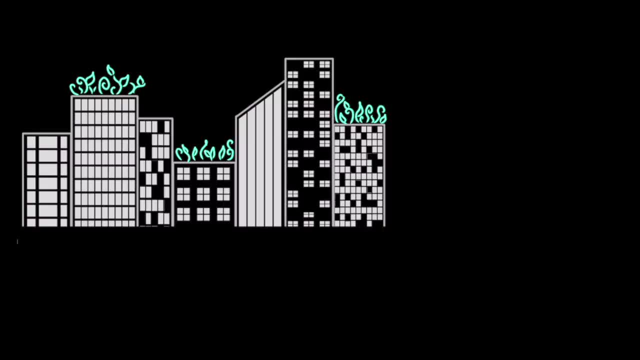 see in the horizon line of cities, And it can be really harmful to eyes and lungs. So how could urban planners solve this problem? Cities could cluster grocery stores, offices and homes closer together, building up rather than out, making buildings taller rather than wider. This would mean that cities would have a lot more space to live in, and that cities would have a lot more space to live in and that people wouldn't have to travel as far to get where they need. So people could rely on walking or biking rather than fossil fuel consuming vehicles. Cities can reduce vehicle. 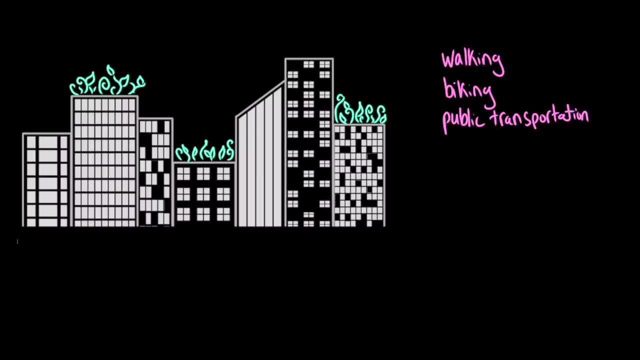 emissions by making public transportation more convenient and affordable. This would mean that fewer people would need to use their own cars to get around, and it would cut down on traffic. Also, cities could build more paths, sidewalks and bike lanes, so people wouldn't have to rely. 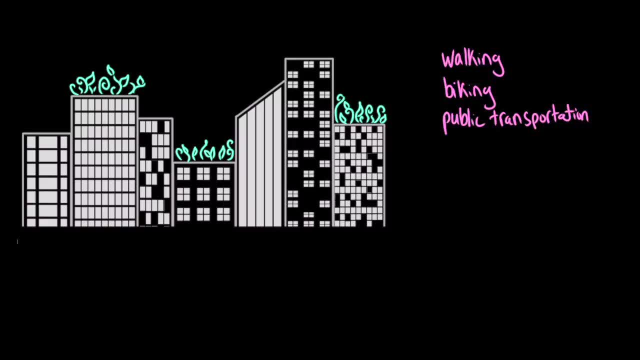 on fossil fuel consuming vehicles to get around. Encouraging walking and biking could also improve the health of city residents. Cities can use clean forms of energy like solar or wind power to reduce air pollution. They could also use fossil fuels more effectively. 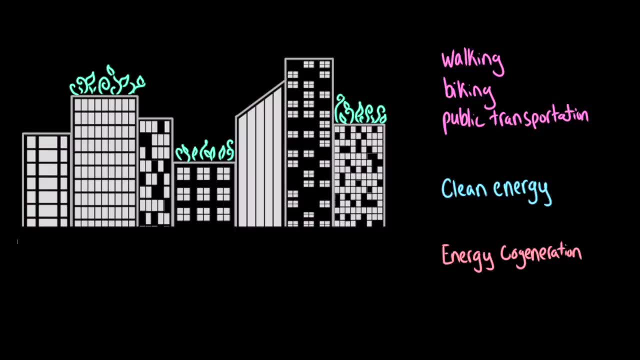 through energy cogeneration, which is a way of using the heat given off by the burning of fossil fuels, not just the electricity. By creating goals and sustainable plans, cities can help reduce air and water pollution and increase the well-being of their residents. The city of Espoo.